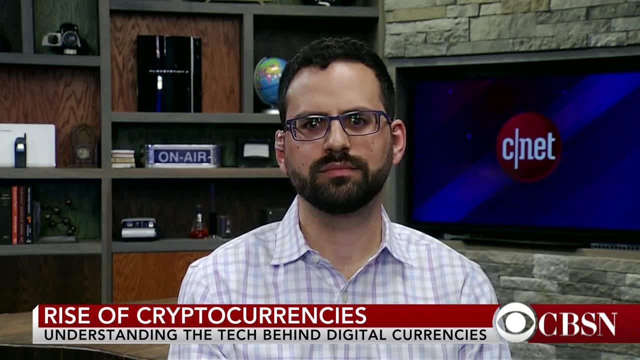 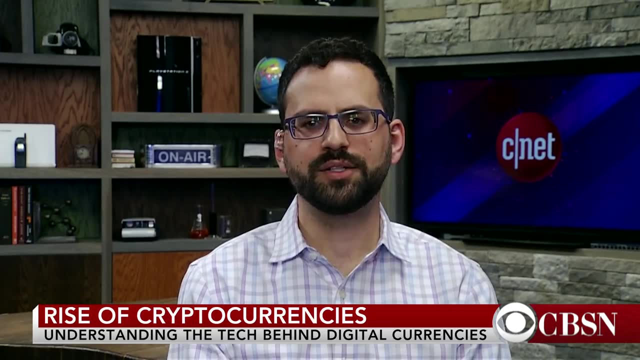 He joins me now from their CNET studios in New York City to discuss it all. Okay, Ben. so for people who really aren't familiar, can you explain the difference between Bitcoin and blockchain? Yeah sure, Bitcoin is essentially an all-virtual currency and blockchain is the technology that. 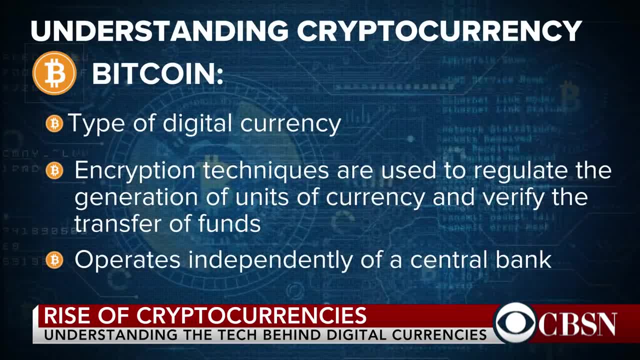 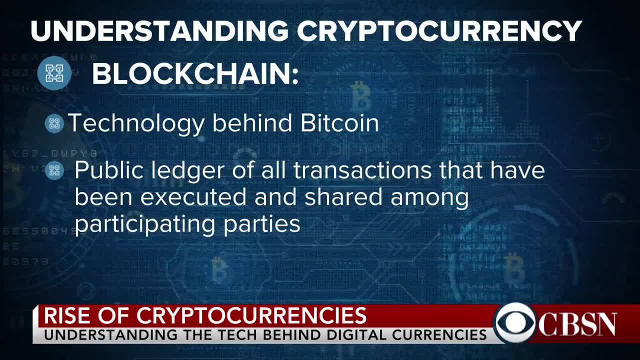 underpins it. Blockchain is a little bit more complicated. It's essentially a giant spreadsheet that's shared throughout a number of computers and once new information is added into it, it can't really be changed. The reason that's important is that it's supposed to increase and 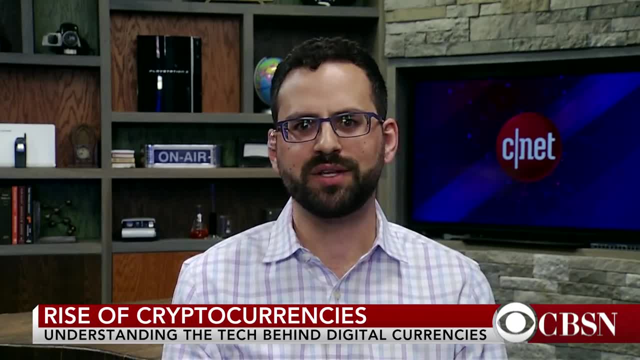 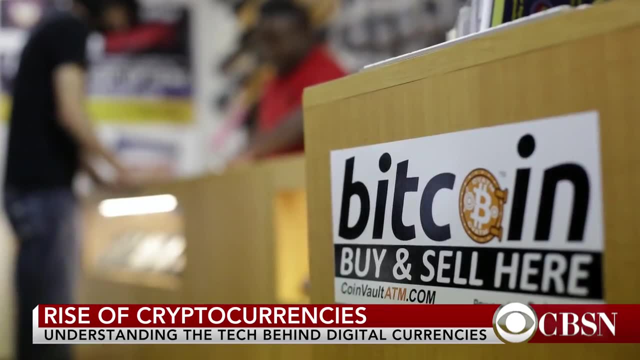 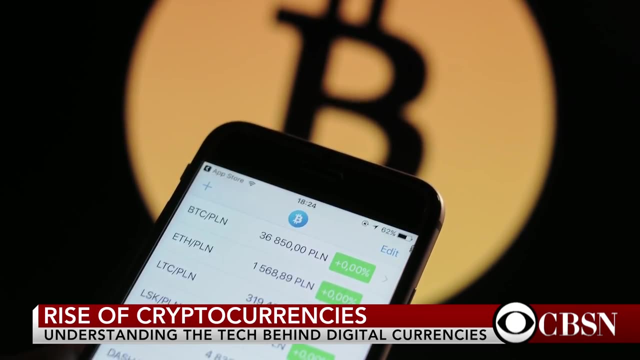 add trust and transparency among different players that might not actually know each other or never actually meet. So how are people using Bitcoin right now? So the promise of Bitcoin was initially that it would replace something like the dollar and the euro. Everybody would actually use it in the future for all sorts of transactions. Unfortunately, 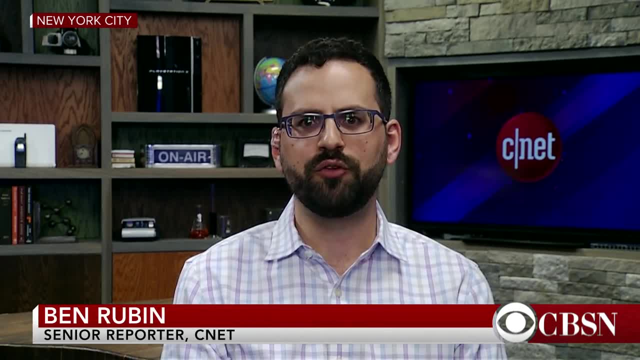 that hasn't really happened yet. It's essentially used mostly for investments, where folks will buy it and then not actually spend it at all. They just kind of keep it as a store of wealth. It's also been used by criminals and fraudsters in a variety of ways. 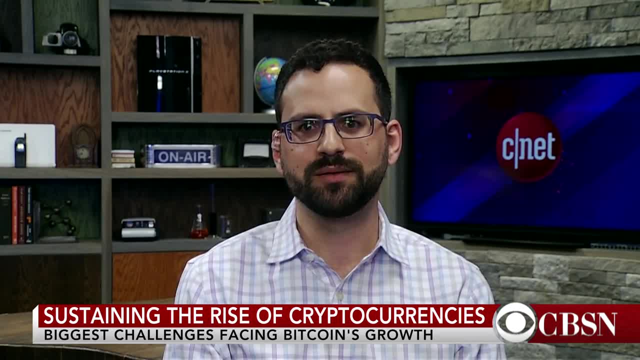 because Bitcoin- Bitcoin itself- can be used anonymously. So you mentioned fraudsters using this. What are the other problems that Bitcoin's encountering right now? Yeah, there are probably three other central problems for Bitcoin right now. First, transaction times can take a really long time. 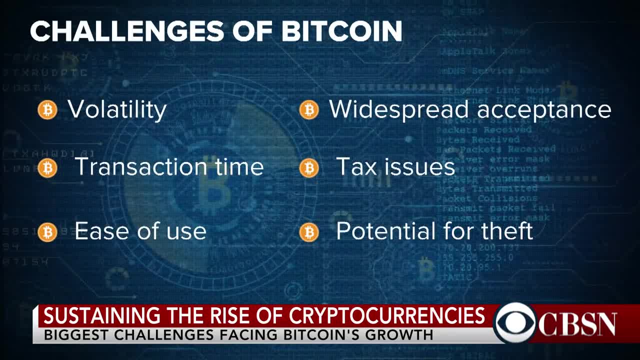 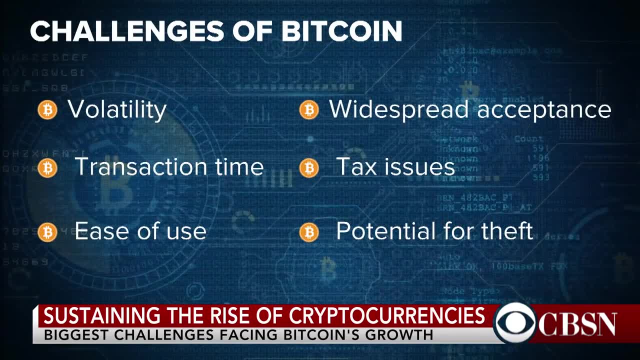 Obviously, if you want to buy a salad and it takes 15 minutes for the transaction to clear, that's a big problem and people wouldn't actually want to use it. Bitcoin also requires an enormous amount of power for those transactions to go through. And the last is that 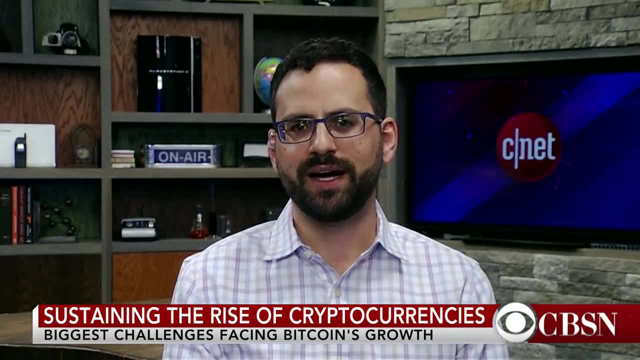 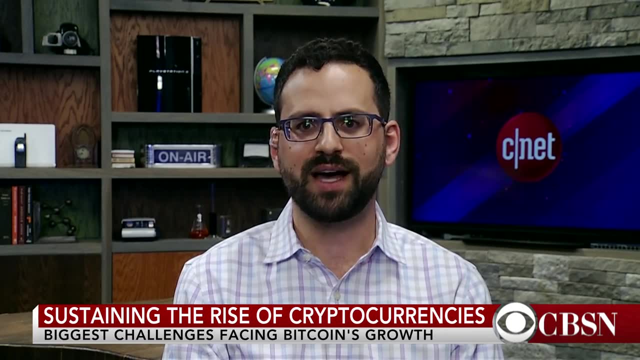 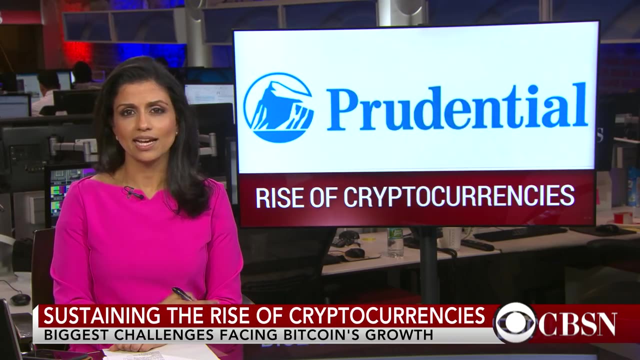 Bitcoin is incredibly, incredibly, incredibly volatile. so during the run up and a lot of excitement for Bitcoin during November and December, it was as high as almost 20,000.. Now it's roughly half that amount. So if you see Bitcoin and other cryptocurrencies have these kinks, do you think that at 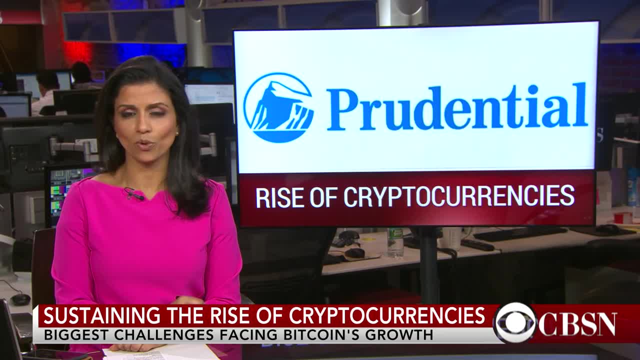 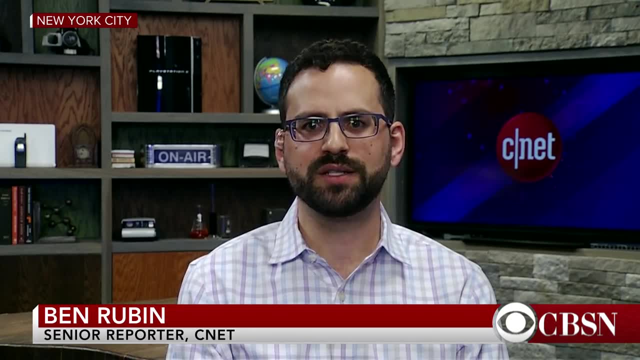 some point. regular folks, everyday folks, will be using it at some point in the coming years. It's certainly possible. there are some efforts to try to iron out some of these problems, Because a lot of the folks that really believe in these crypto, cryptocurrencies, and see them as the future, want to solve these problems. And if they do, in fact